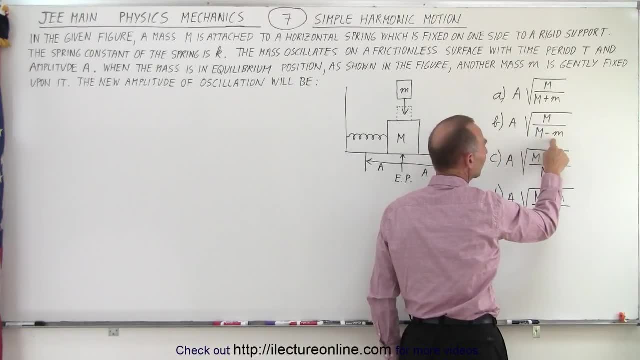 But here notice that when you divide M by M minus M, that's a number that's greater than one. so definitely B could not be a possible answer Here. when you look at M minus M over M, this is less than one. so this could be a possible answer. 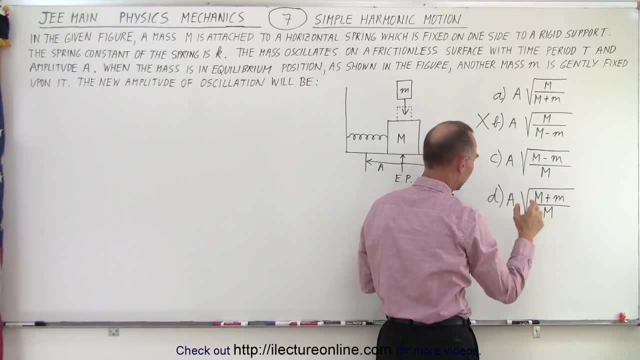 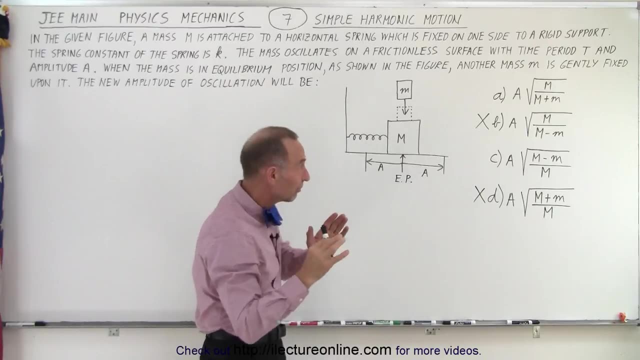 But here M plus M over M, that's a number bigger than one, and again this is not possible. So right away, if you don't know how to solve this problem, at least from the perspective that the amplitude has to become smaller, you can already eliminate two of the four answers. 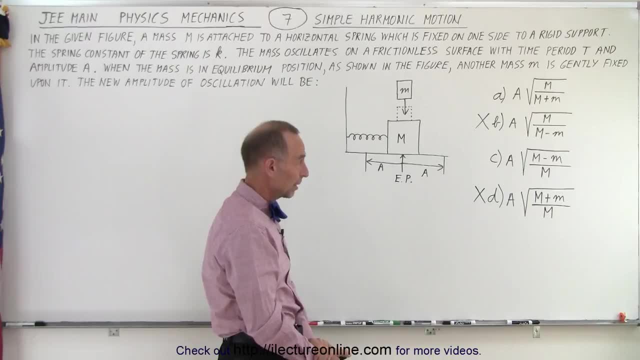 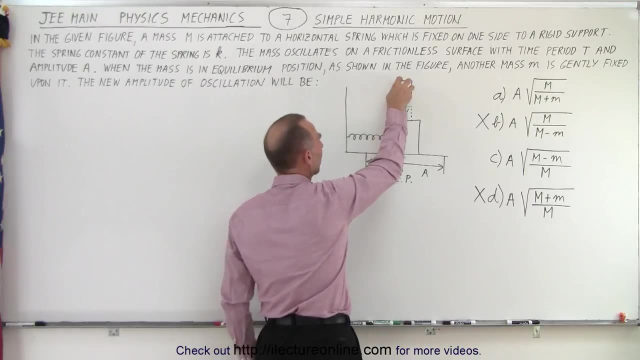 and now you have a 50-50 chance of guessing the right answer. All right. next, How do we approach this? What is the concept here? Now notice, when you place one object on top of another like this, that's kind of like a collision. So whenever you bring two masses together, 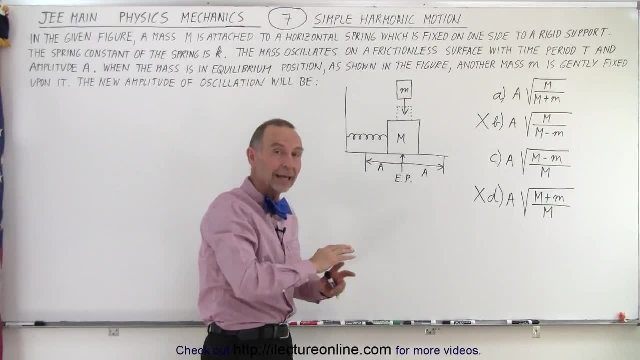 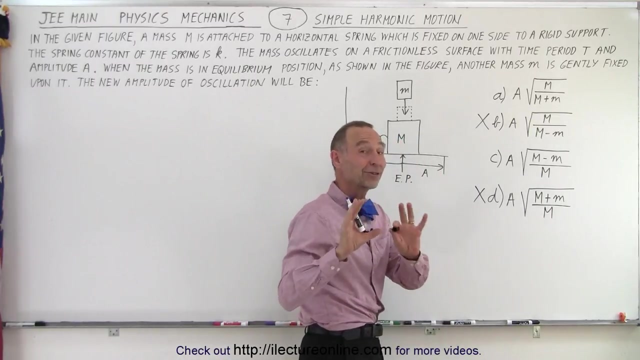 one thing is always conserved, which is momentum, and the other thing is essentially never conserved unless it's a perfectly elastic collision, and that would be energy. So the principle of conservation of energy is key to solving this problem. So conservation, oh not energy, conservation of momentum. 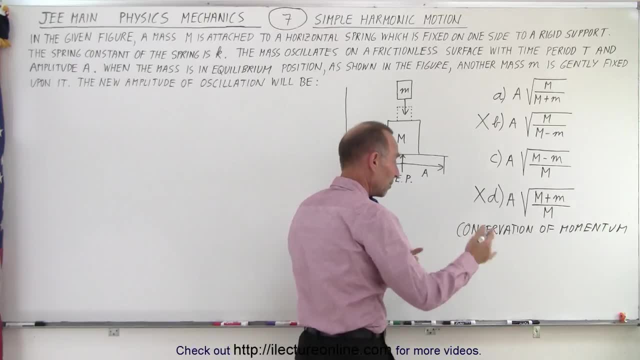 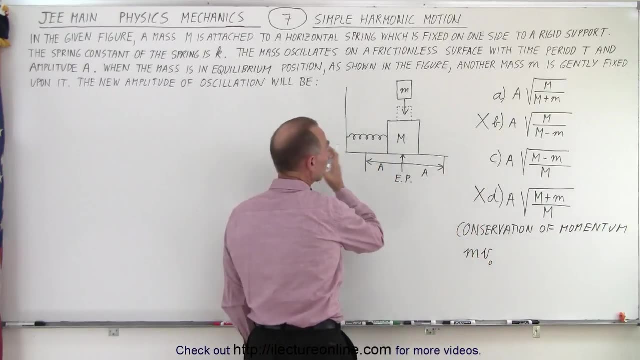 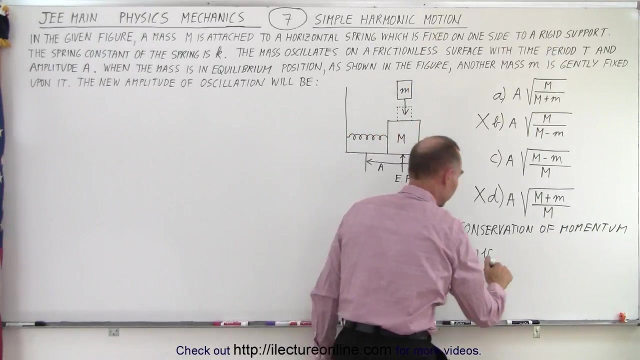 So if we use that principle, what do we get? Well, that means that the momentum before equals momentum after, So the small mass times its initial velocity. but notice, we only care about the velocity in the x-direction. so the small mass had no velocity in the x-direction initially, so that goes to zero. 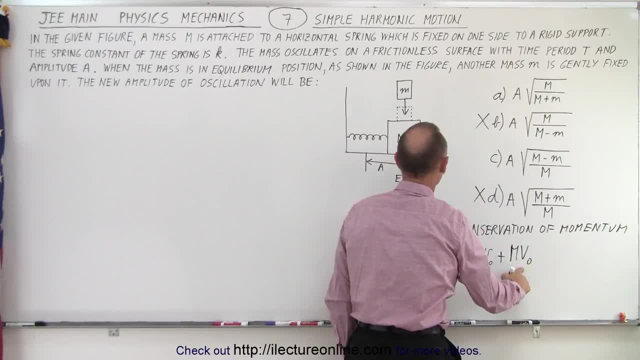 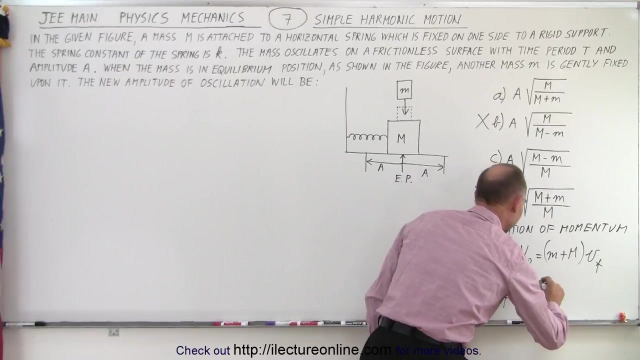 plus the big mass with its initial velocity. That must equal the sum of the two masses with the final velocity, and of course this goes to zero, which means that the final velocity is equal to the initial velocity, times m divided by m plus m, like that. 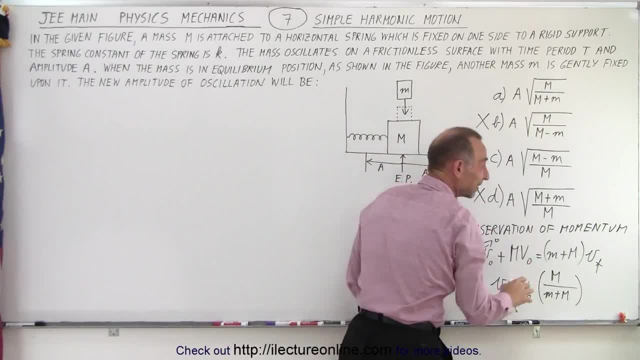 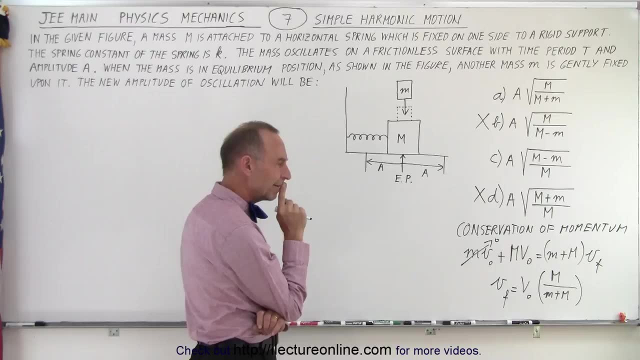 And then you take a look at these possible answers and you go: well, maybe that's one of them, but that would be a stretch to make that decision at this moment in time. So what we can then say is that our energy, our maximum energy, E max. 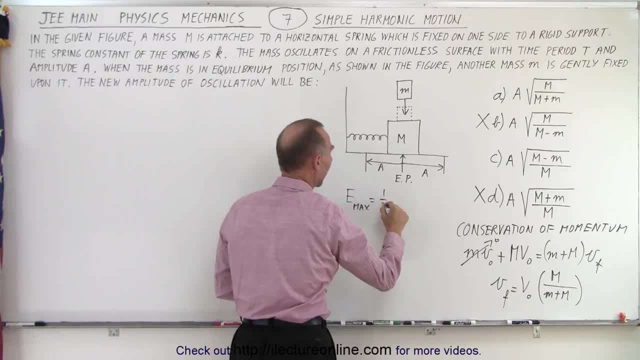 before we add, the small block is going to be equal to one half the big M times v max squared. So that would be the velocity at the moment that the block goes to the equilibrium point, which is when you put the small mass on top of it. 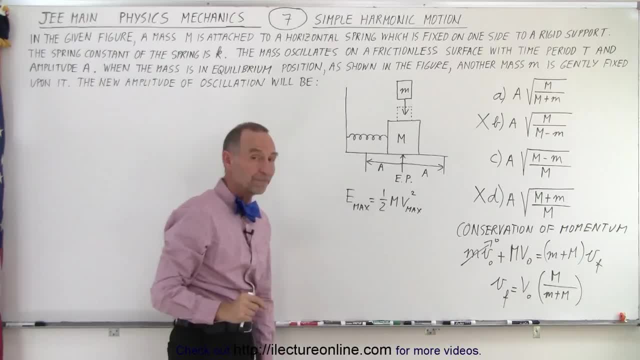 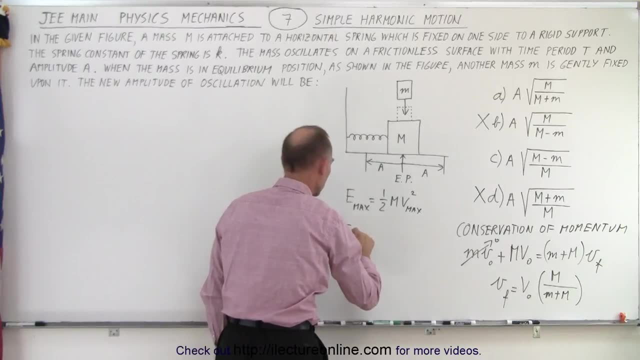 So that's the initial maximum energy Once you put the small block on top of it. what happens now is that E new is going to be equal to one half the new mass, which is m plus m. and let me write the big M first. 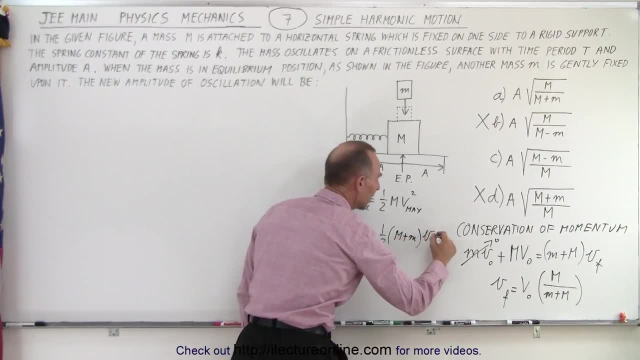 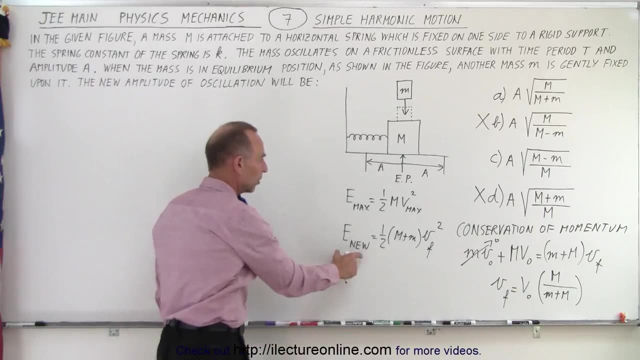 big M plus small m times v, final squared. So we know that the new energy, which is going to be less than the maximum energy we started with, is going to be equal to this. We end up with a smaller velocity because- notice that this is a fraction smaller than one. 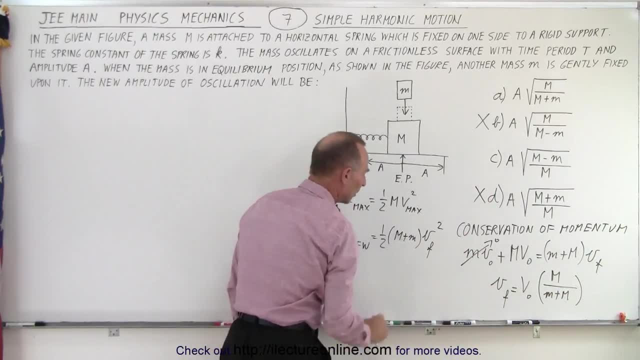 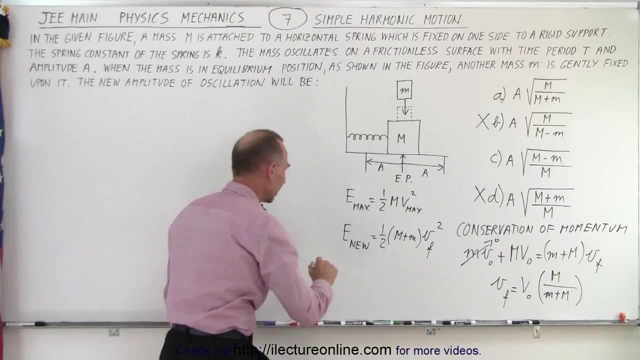 so we end up with a less velocity and we end up with more mass. Next, because we're dealing with the amplitude, we can also say that the E new is also equal to one half k amplitude new squared Right, because afterwards what happens is we have a new mass. 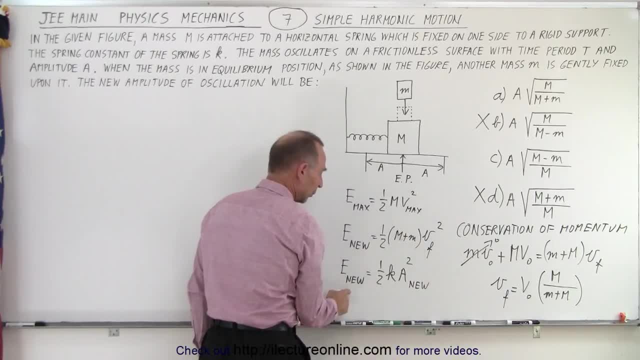 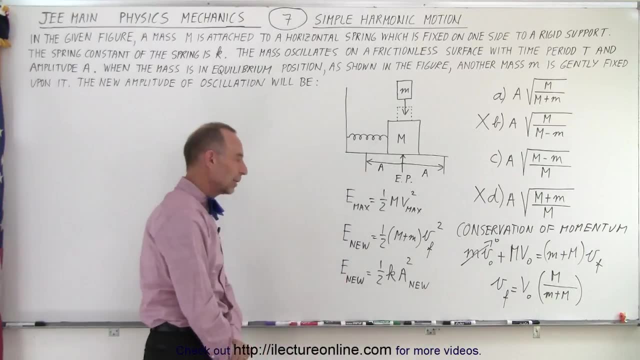 oscillating back and forth with a new maximum velocity, and that will then give us the equivalent potential energy stored in the spring, when it's completely collapsed at the maximum amplitude. So we know that those two have to be equal to each other. Okay, now it becomes a little tricky. Where do we go next? 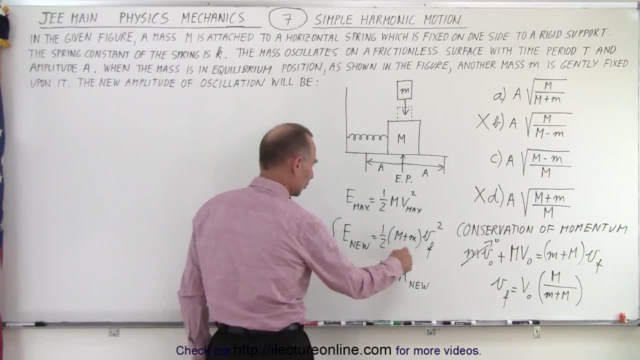 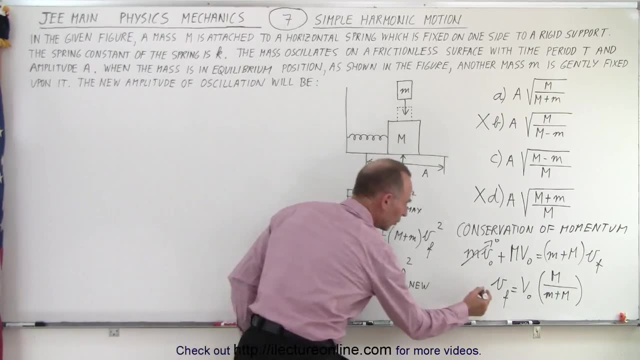 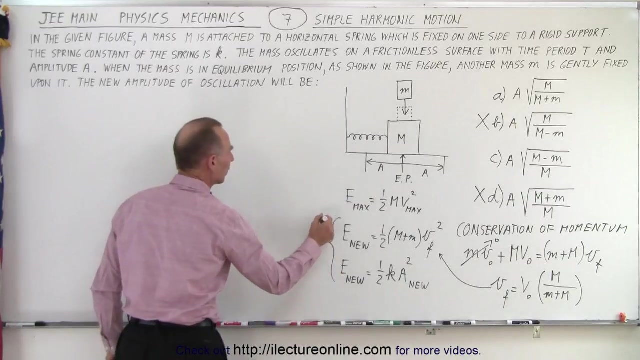 Notice: we have the new energy in terms of the kinetic energy, we have the new energy in terms of the potential energy. but what we should do right first is this Notice that we have V final expressed in terms of V initial and the ratio of the masses. 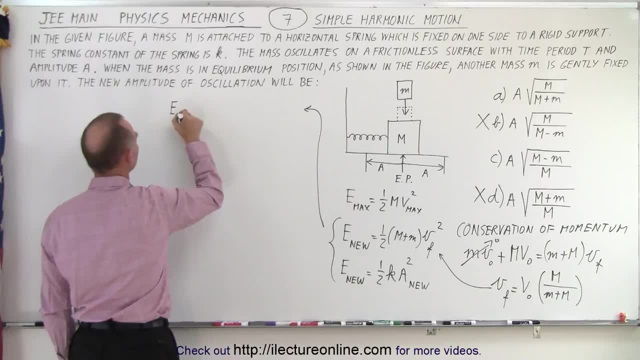 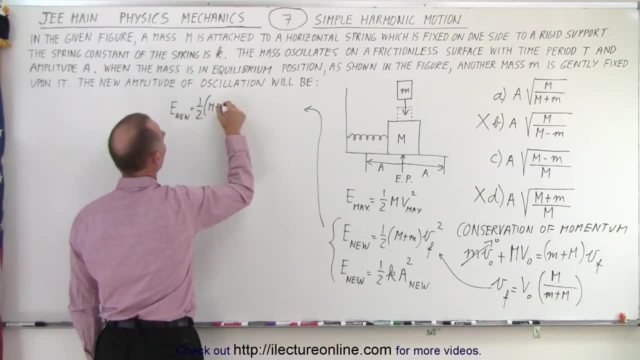 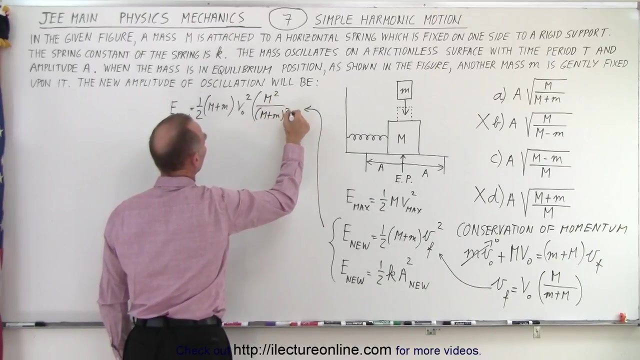 So what we're going to do is we're going to then write an equation for e new, which is equal to one half m plus m times V initial, and that has to be squared. oops, that should be a 2, squared ratio of m squared and m plus m squared- and then simplifying that this cancels out with one of. 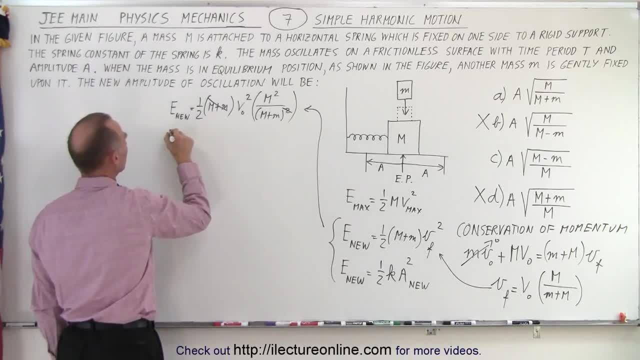 those and then notice that we could write this e new as one half m v, initial squared times m over m plus m. so notice that the new energy is the old energy because that's the original energy. that was the original velocity and the original mass. so the original energy times a fraction less. 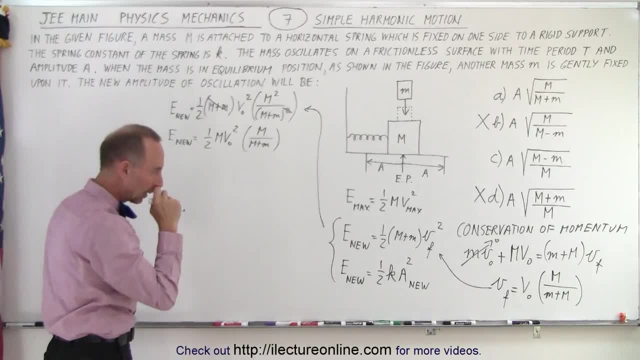 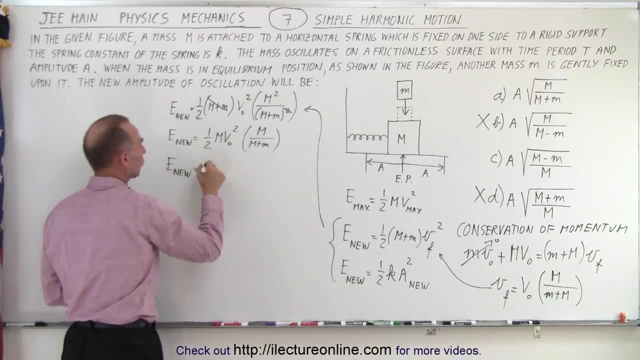 than one. so now the new energy is less than the old energy. so we can do the same for the potential energy. we can say that e new is equal to the old energy, which is one half k a squared, where a is the original amplitude, times the ratio. oh k a squared, yes, times the ratio of m over m plus m. 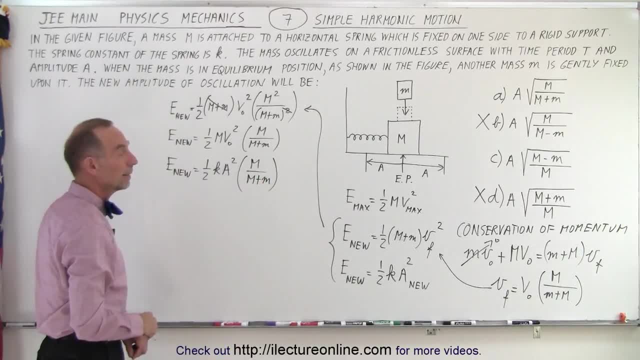 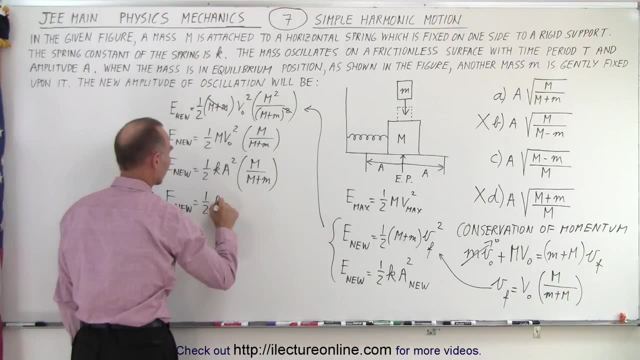 okay. now if i write it like this: e new is equal to one half k, a squared times the square root of m over m plus m. squared like this, then you can see that a new must equal a old times the square root of M over M plus M. and so now I have found the relationship by: 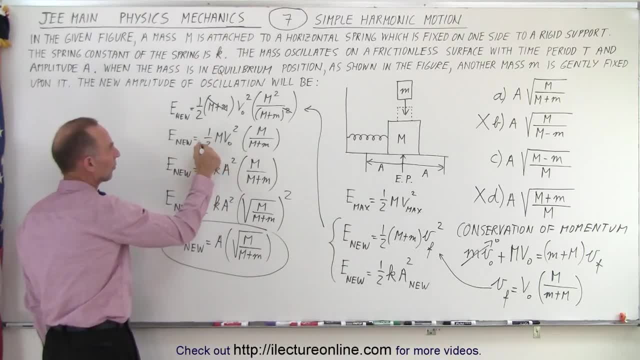 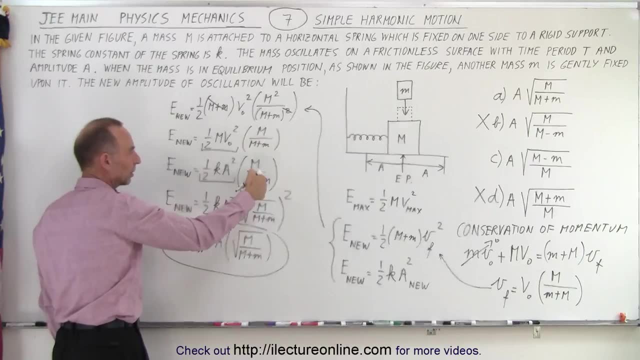 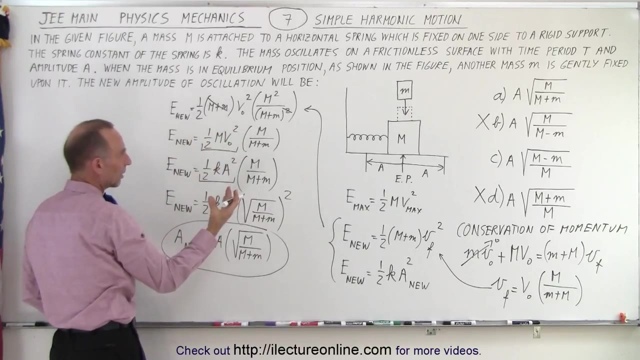 first comparing the kinetic energy, new to old, because this is the old kinetic energy, and then I go to potential energy. this is the old potential energy times, of course, the same ratio, because the same fraction, because the total energy has changed. either way, if I use kinetic or potential energy, it doesn't matter. 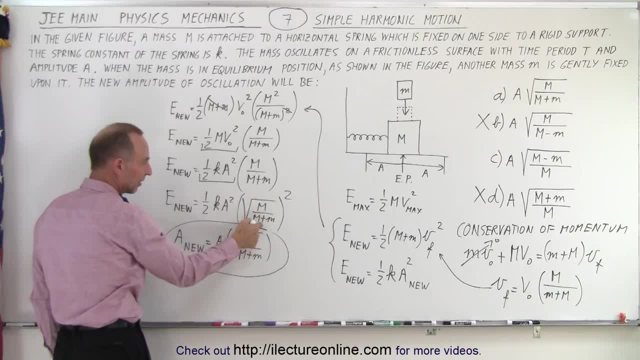 then if I realize that if I write this like this, then I can pull out the a new which is a old times, this fraction, the square root of that, and then we come up here and then we realize that answer, a one of the two possible answers, end up, 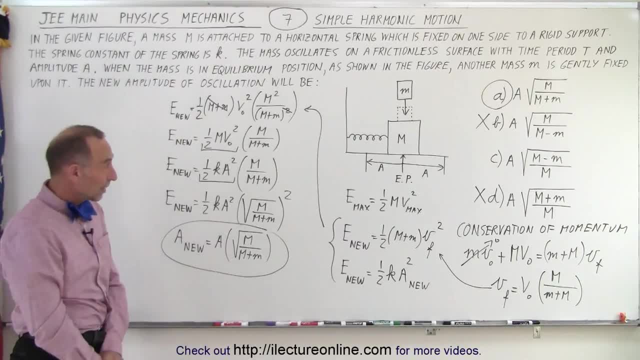 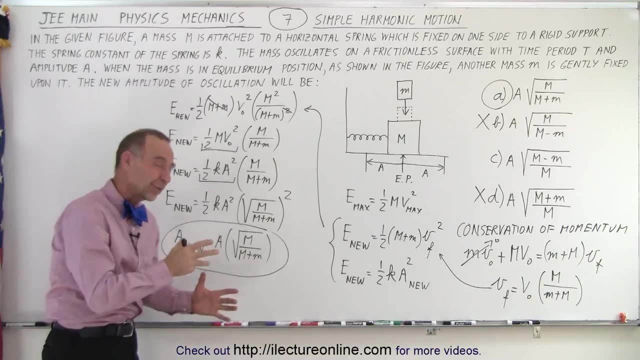 being the correct answer. so yes, it's these types of problems, especially with simple monic motion, when you change something and then try to find the changes something else. they're usually mind changing. they're usually mind twisters, no matter how they're phrased. there's lots of different ways we can. 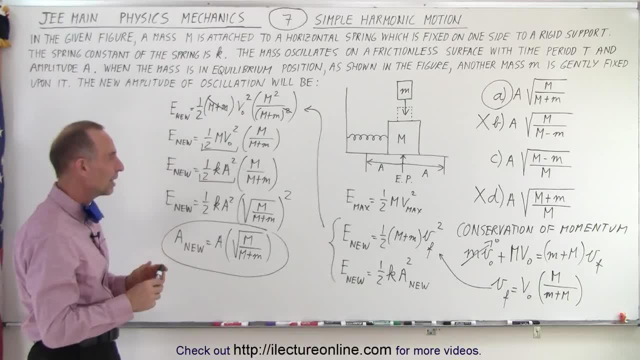 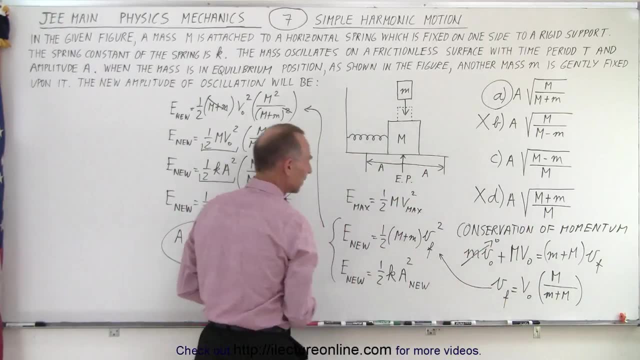 phrase that it kind of makes it difficult and you always have to go back to the basic principles that you have, first of all, conservation momentum to find the new or final velocity, then realizing that this was the original energy. the new energy is then going to be defined by a new mass and new 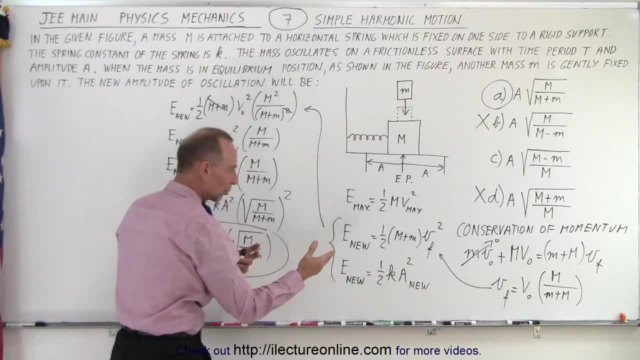 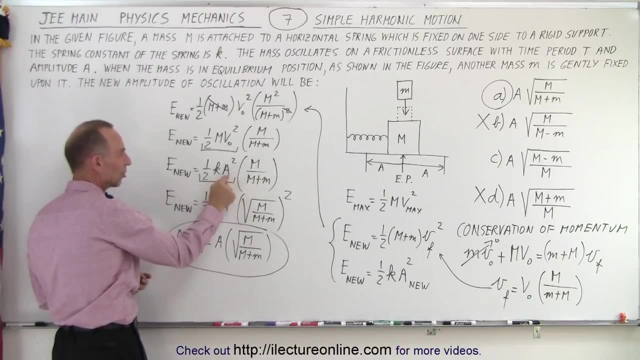 velocity, which is defined here and now. we have to find the relationship between the old energy and the new energy, both in terms of kinetic energy and potential energy. and finally, once you have the change in the amplitude, realizing that a times the square root of m over m plus m, then you 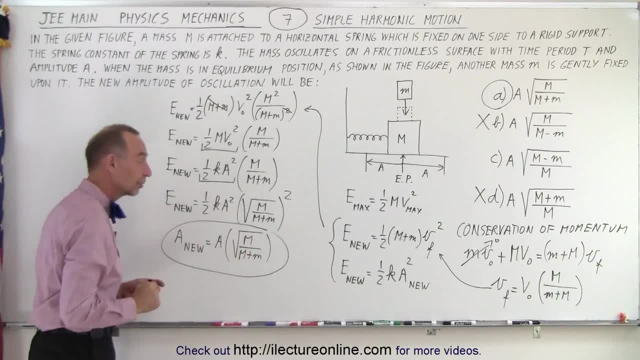 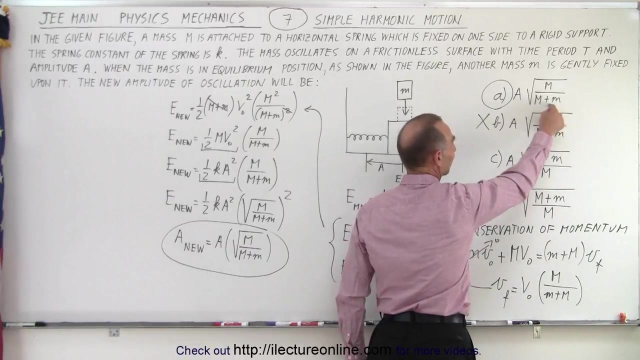 have the new amplitude defined in terms of the old amplitude, and that is how it's done. um, yeah, yeah, right from the beginning, when i had this relationship here, i was leaning very much to saying that's got to be the answer because of the way the the ratio of the masses were. 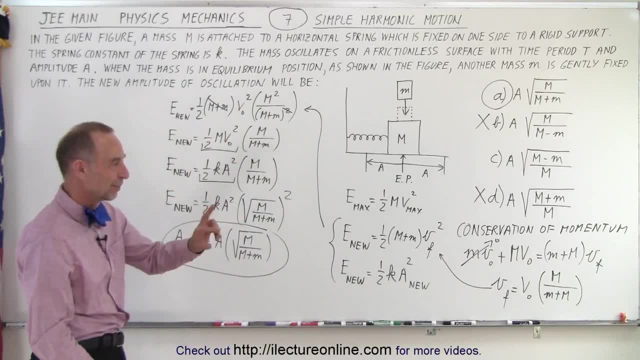 were positioned there. but again, it's a leap of fate. maybe it's, or maybe it's the inverse, you don't know right. once you substitute it in, then you know that it's not going to correct. once you substitute it in and it's even like this, you realize that it's probably going. 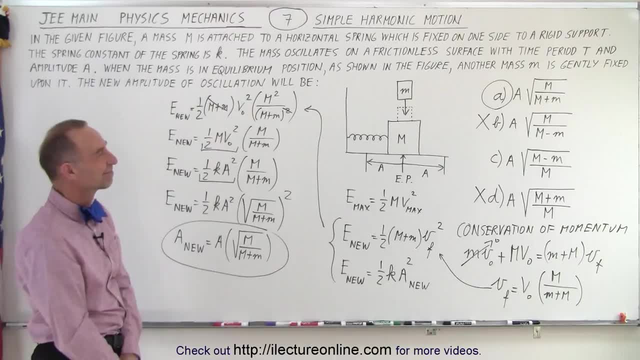 to be that ratio right there? yeah, you're not. you realize you're not going to be able to move it to the other side of the equation and even if you do, the other one is m minus m. yes, you realize that this is always going to be on the right side equation. you're already half your. 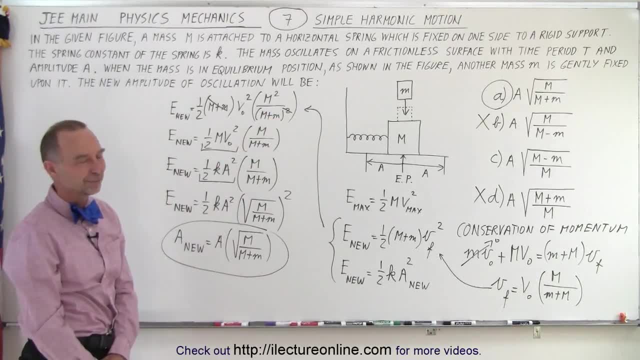 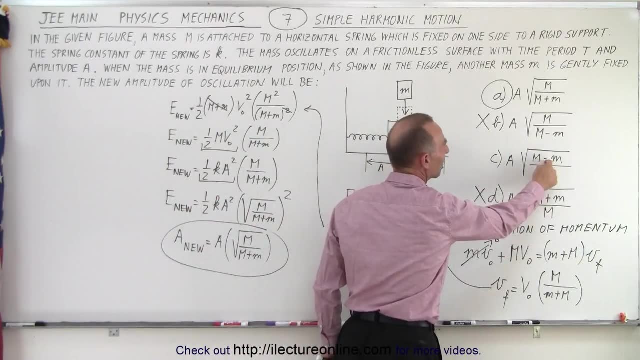 ratio. so you probably want to go through a leap of faith: m minus m. this one's m plus m. well, the minus could not. this could not be, this could not be correct. oh, and here's m minus m. so, yeah, that's also a very unlikely scenario. so, yeah, you probably don't need to work all the way through in order to. 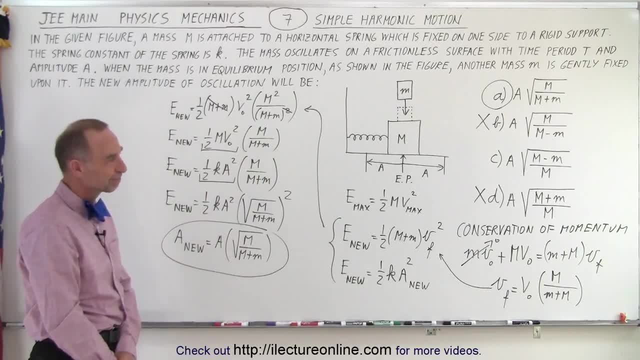 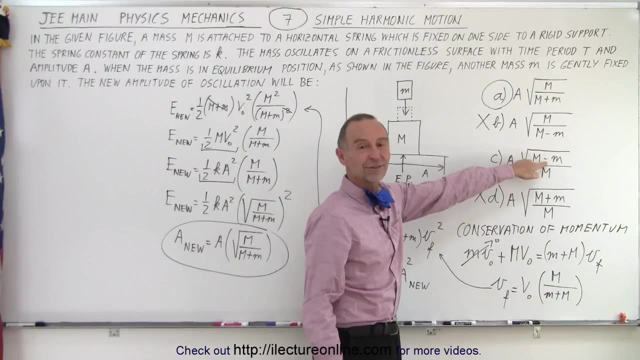 show that you got the right answer. so that's how you always know: save a few seconds here if you're a second there, that is true. so first of all, you could quickly eliminate these, and then you want to eliminate this because the minus, because you end up with this, yep, that's probably good enough. 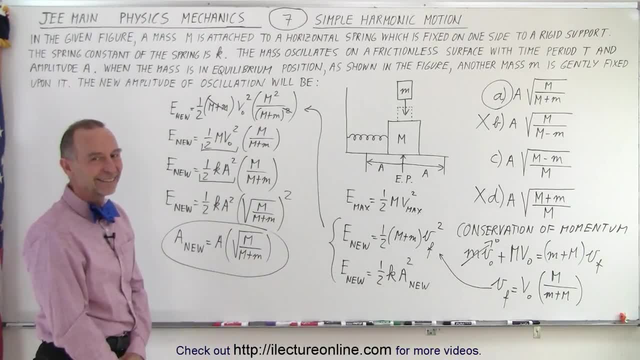 yeah, that's how you save yourself for the other five minute, seven minute cycle, because then you run out of time at the end and you can't do all the problems. so you want to save time. so this was probably not even necessary. simply by realizing conservation momentum you have. 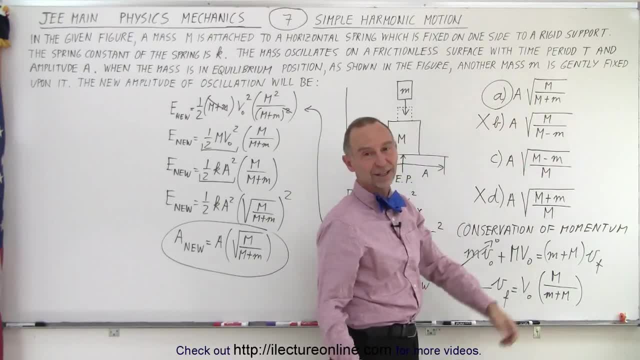 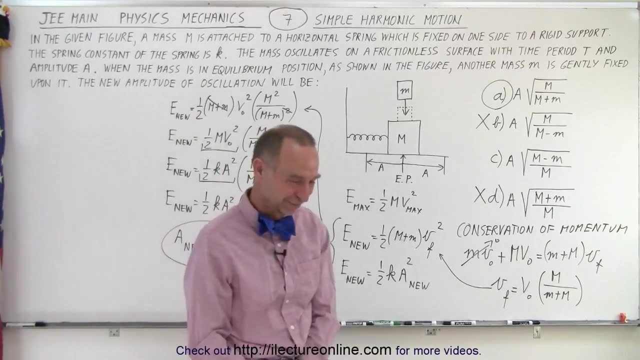 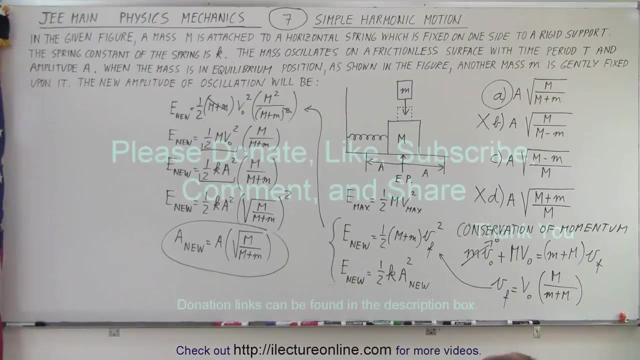 this relationship, so it cannot be this one. it's got to be that one done, move on. yes, I would take my chances on that, mm-hmm. yep, you're right, yeah. 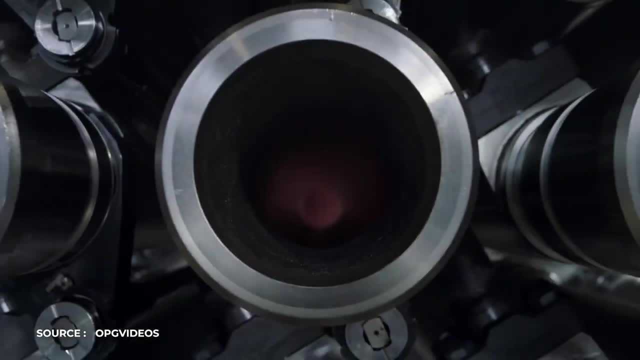 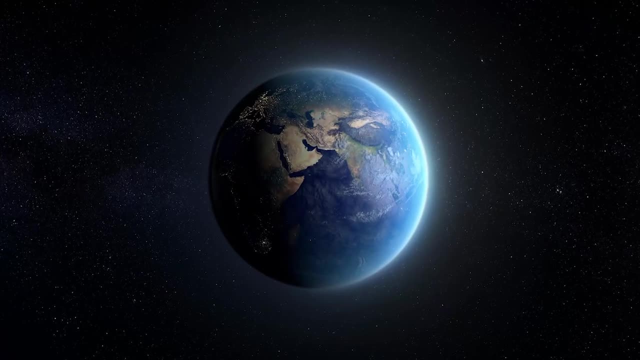 Canada is a tier one nuclear nation, home to one of the world's most innovative nuclear power reactors, known as the CANDU or the Canadian deuterium nuclear reactor. As the world looks towards combating climate change and reducing its emissions, nuclear technologies present a 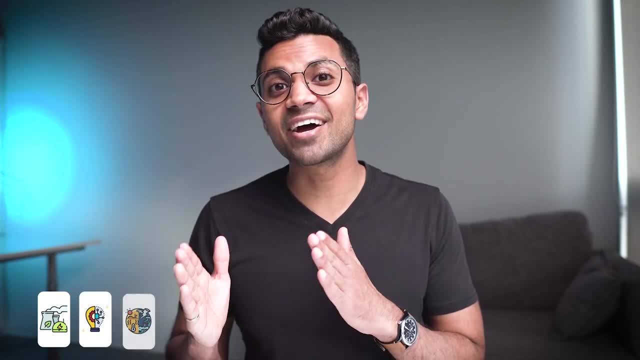 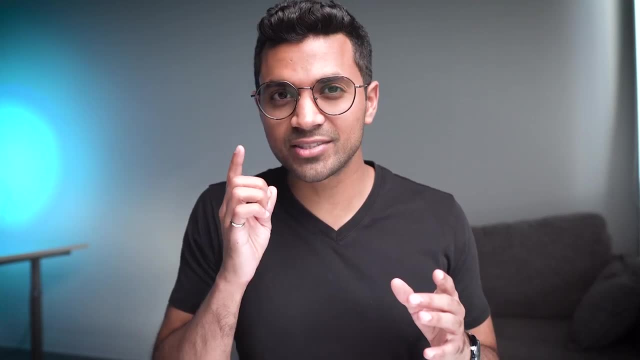 really good opportunity to both advance humanity and mitigate the effects of climate change. That's why, in this video, I'll be doing a technical deep dive into the CANDU reactor and explaining exactly how this nuclear power reactor works. I'll be going through everything you need to know about. 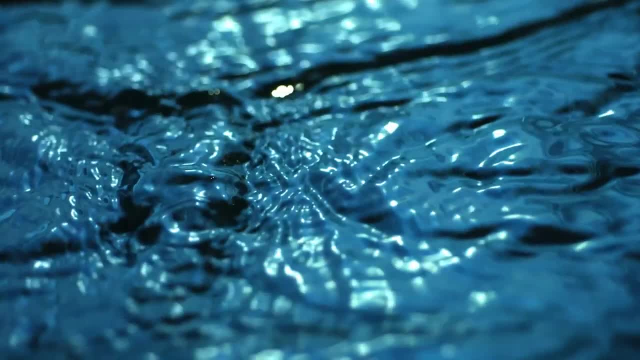 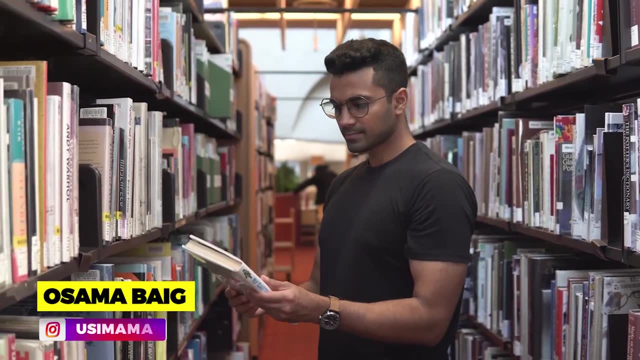 this CANDU reactor design, which is pressure tubes, heavy water, how it takes natural uranium fuel and converts that into electricity end to end. Hey friends, my name is Osama, I have a background in nuclear engineering and on this channel I help demystify nuclear technologies. 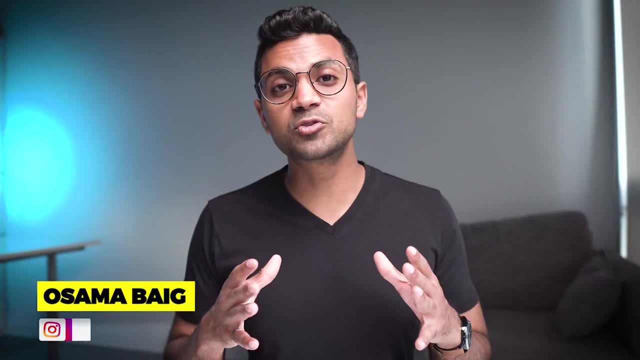 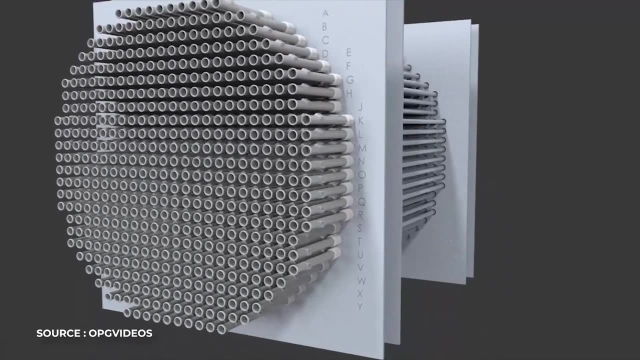 by simplifying them. I also make educational resources on all things related to the CANDU nuclear reactor as well. Let's start with the calandria, which is the heart of the CANDU reactor. It's the reactor vessel which holds the fuel and pressure tubes in this reactor. Imagine a large